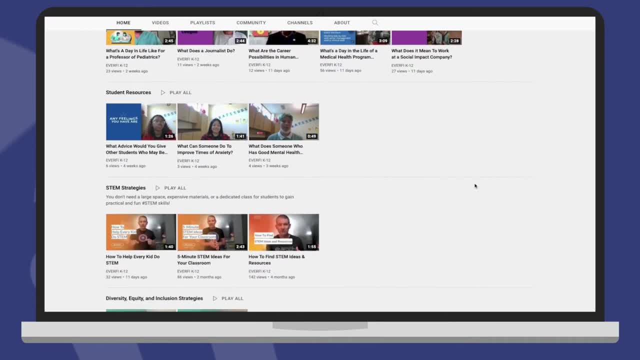 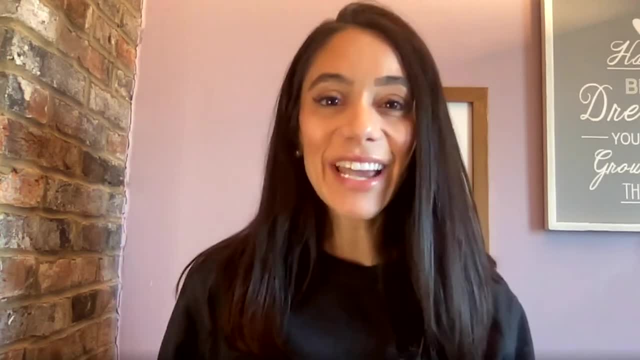 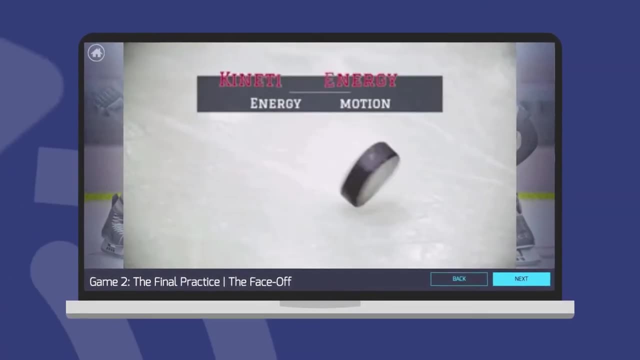 concepts that you're teaching. bring it to life a little bit more. Hear it from other folks. Let that be kind of the teaser for the rest of your lesson. In EverFi's lessons, too, there's a lot of video content. For example, in our Future Goals, Hockey, Scholar lessons, each piece of vocabulary is brought. 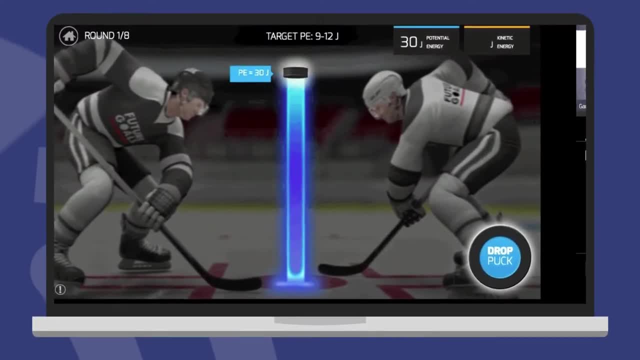 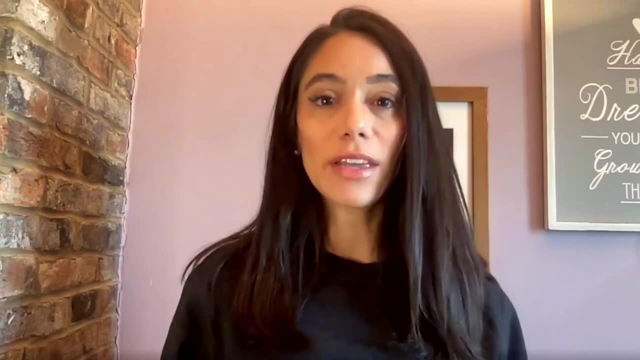 to life through a video, so that folks can, you know, learn a little bit more about what's going on in the classroom. You can see what that vocabulary word is and then watch it in action. How is it applied to real life? I want to elevate student voice. I want to have a different way to gauge student learning. Think of 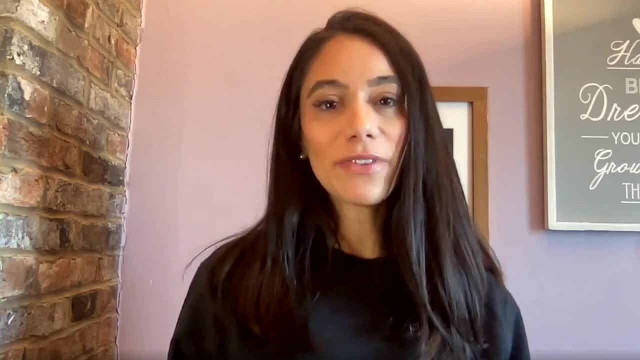 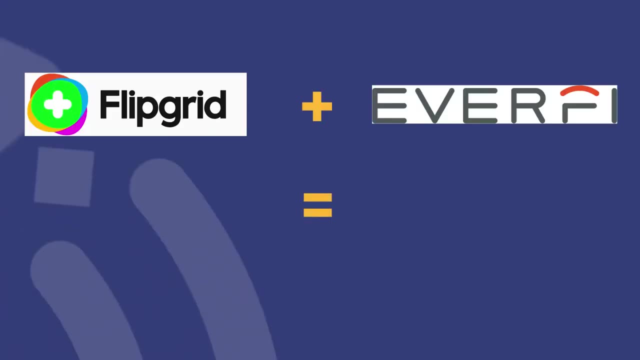 this as your formative assessment in a really easy, fun way for students, And one of the greatest ways to do that is through a tool called Flipgrid. If you haven't checked it out, I encourage you to go. The work that I'm doing here is really free of cost. Students love it, and not only do they get to record themselves. 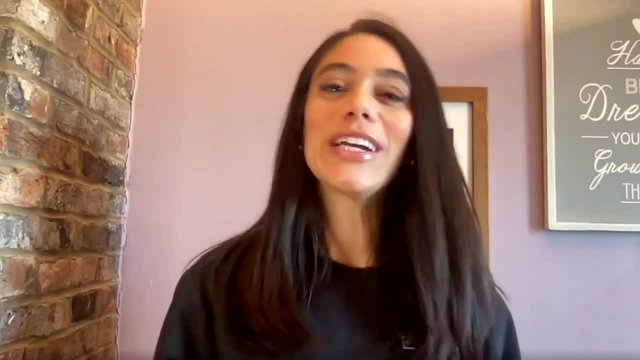 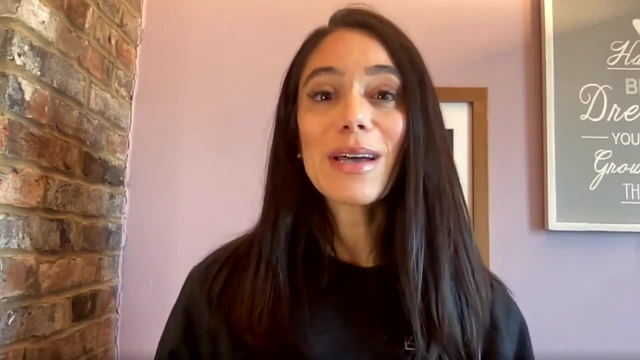 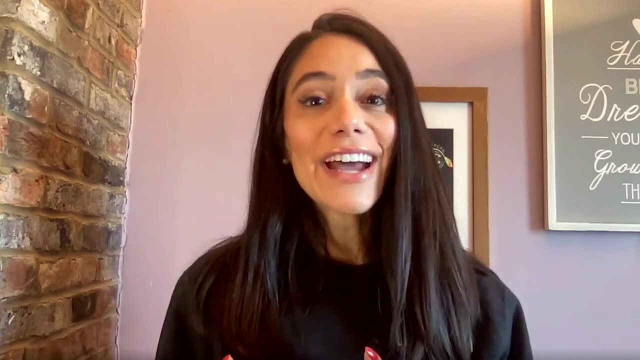 it's almost a little bit like Instagram, where they're creating these videos, that they can provide feedback to you, their thinking, how well they understood a concept Where this applies in real life. Flipgrid is loved by students of all ages. EverFi has a ton of SEL videos that you can. 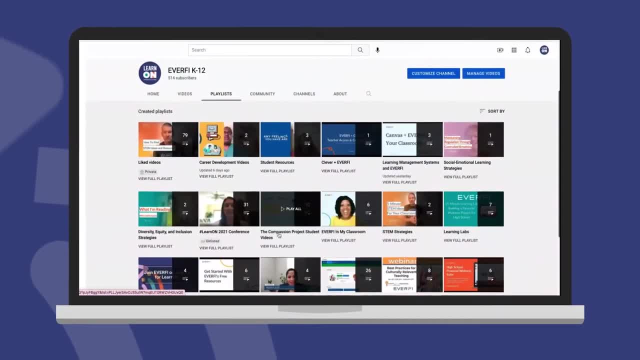 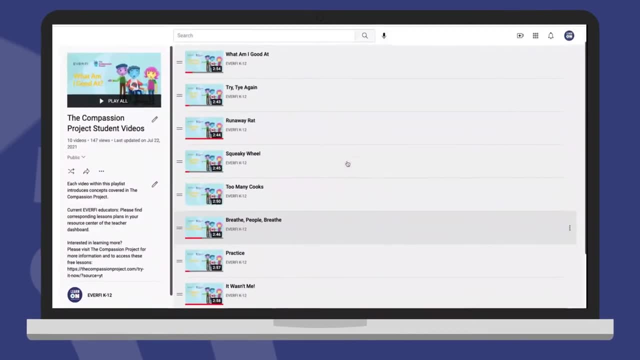 use on Flipgrid as a product. If you're a student who's looking to learn how to live smartly- what you can- If you head over to our YouTube channel, you're going to find a library of videos that go along with the elementary resource, the Compassion Project. 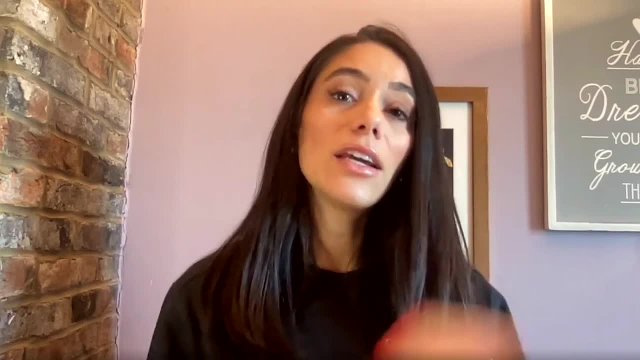 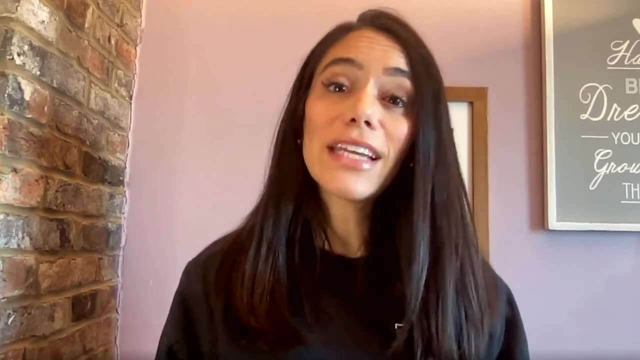 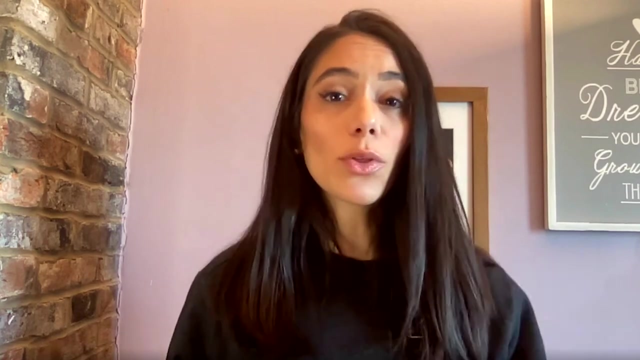 You can have students watch these short videos and then hop onto Flipgrid and they can share about maybe how they would handle the different situation, Have they encountered it in their real life. This could be used for your secondary students as well. Have them work through one of the EverFi lessons and then reflect back on what they learned. 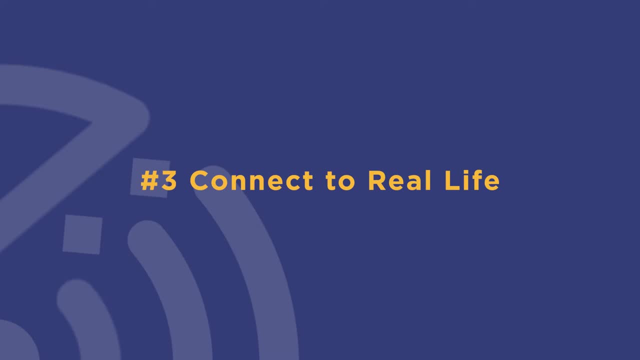 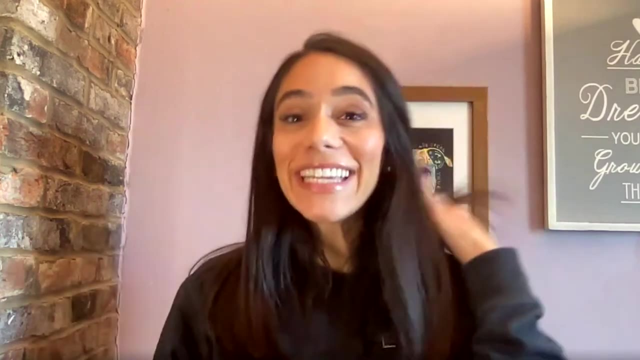 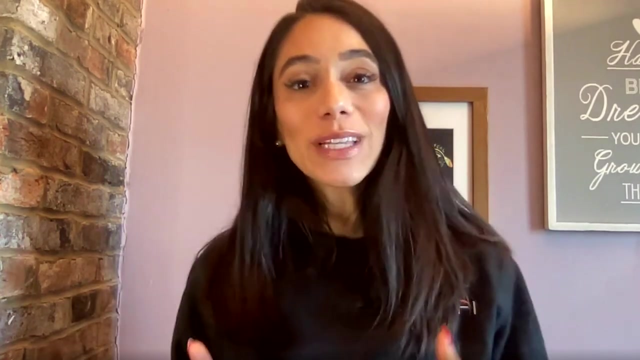 Strategy number three is always connecting back to real life. We know the age old question: when am I ever going to use this? Totally eliminate that from your student's vocabulary. One: the EverFi lessons are all related to real life concepts. The students are going to see characters. 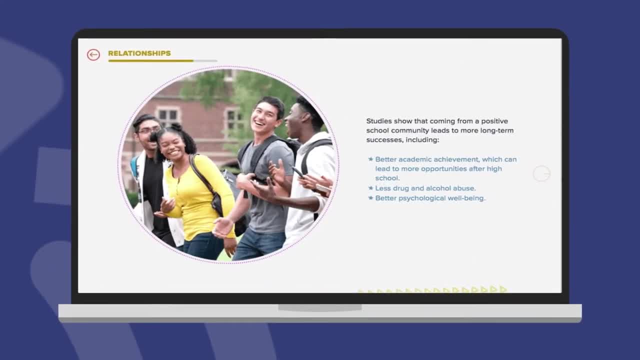 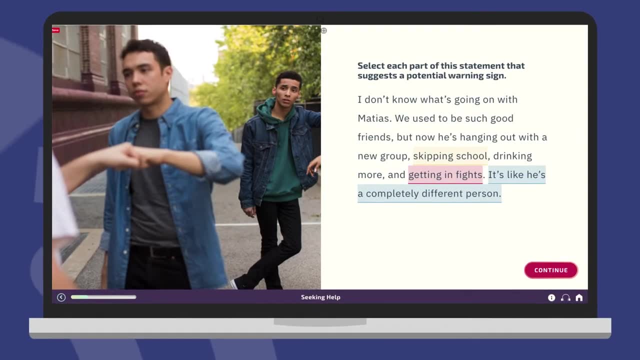 They're going to hear stories. They're going to hear students' stories. but take that and expand upon it. Bring some guest speakers into your classroom, or even share your own stories. What was it like when you went through school? How did you search for it? 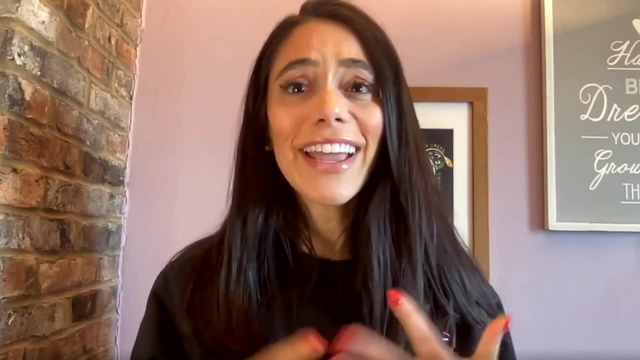 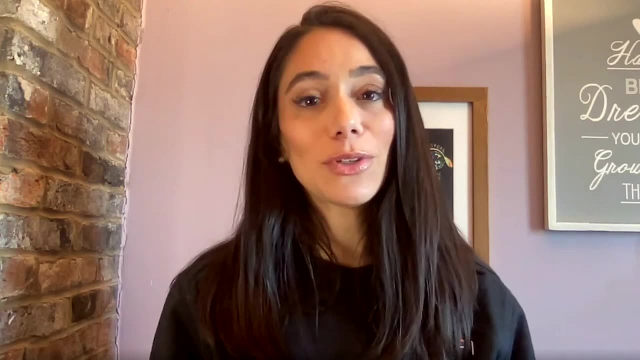 What scholarships did you apply to? What was the loan process like? How do you fill out a FAFSA form? It's all about those connections and creating that relationship with your students, And this is another way to do so. And lastly, engagement strategy number four. 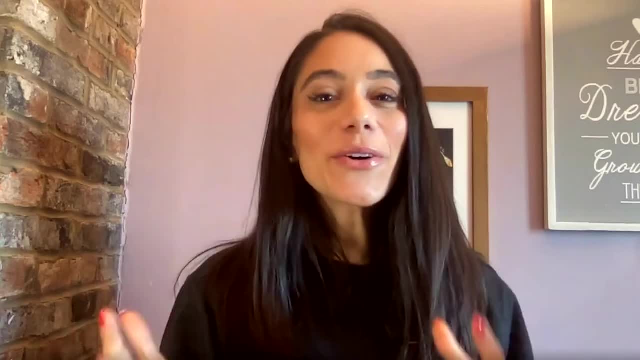 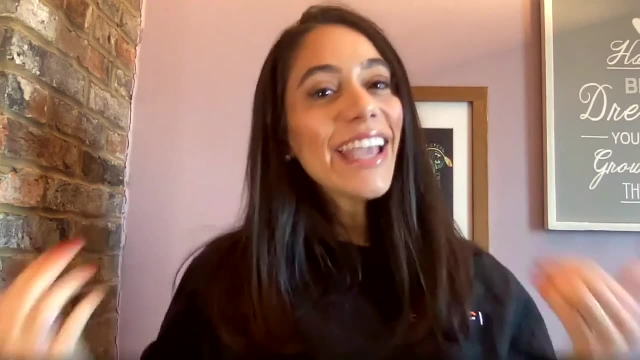 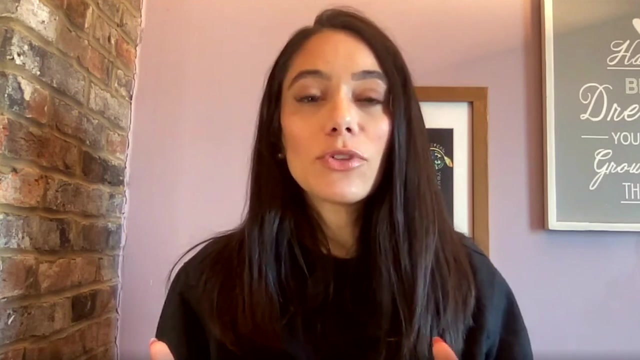 Is build a project. There's always something that you can make with your hands. that was related to this right. Get up out of your seat. Yeah, I love some videos, but let's go create a video on our own, Or maybe there's a STEM strategy that I'm trying to teach. 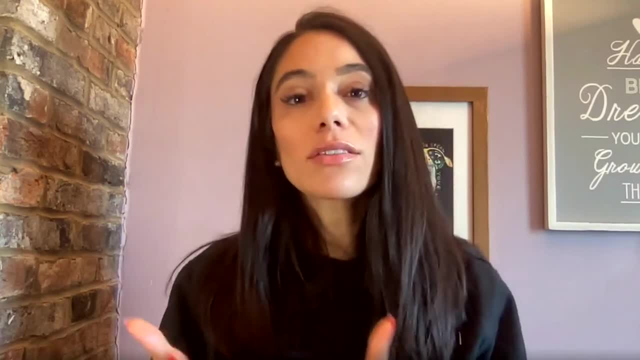 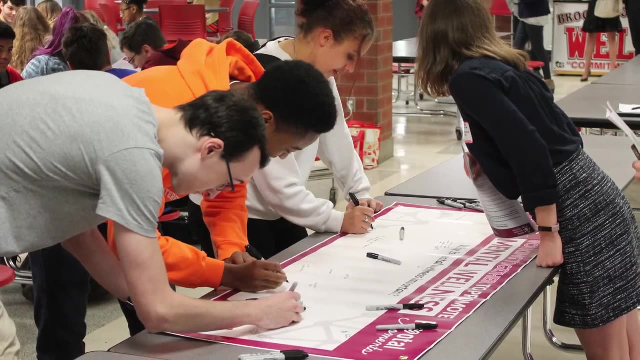 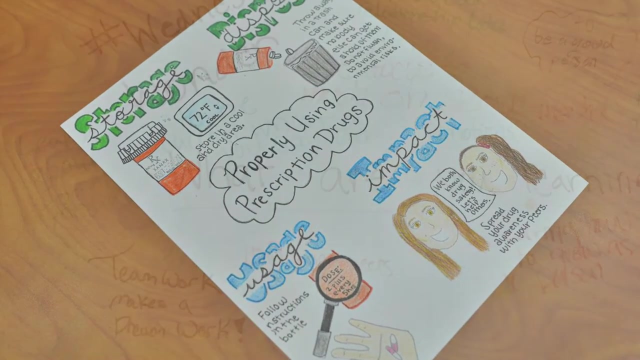 But I want students to actually walk through the process of how that works. So there's a couple of different pieces here in EverFi that's going to be pre-made for you. Everything is there for you. Everything is there for you So that if you have maybe a PSA contest around health and wellness, you want your students to complete. 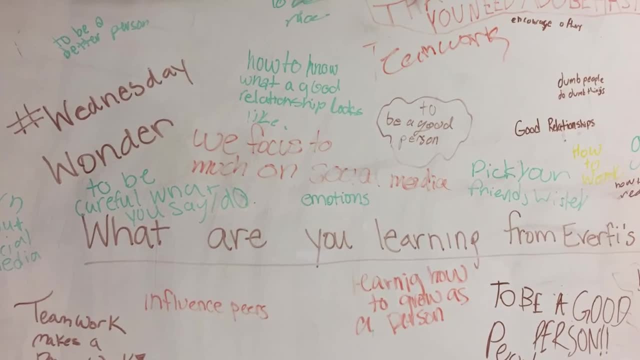 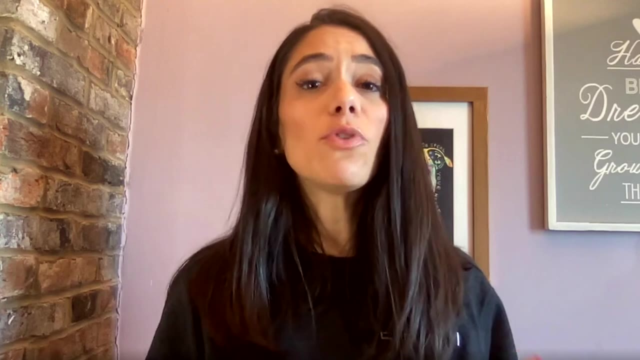 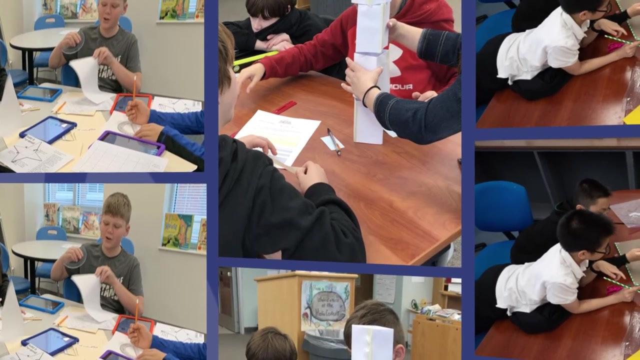 grab that lesson out of EverFi's resources. Have the students use their video editing or maybe create some flyers for around the school where they're informing others of the health strategies and concepts that they have learned. There's student labs in our STEM programs. 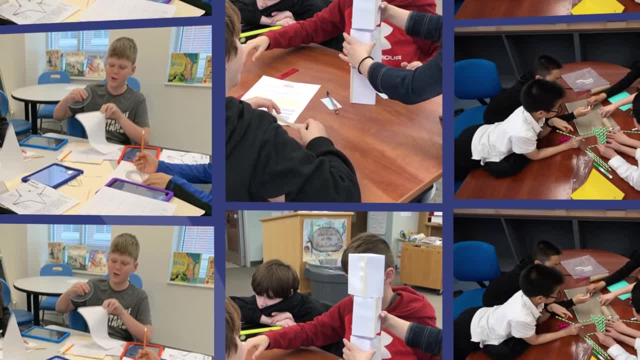 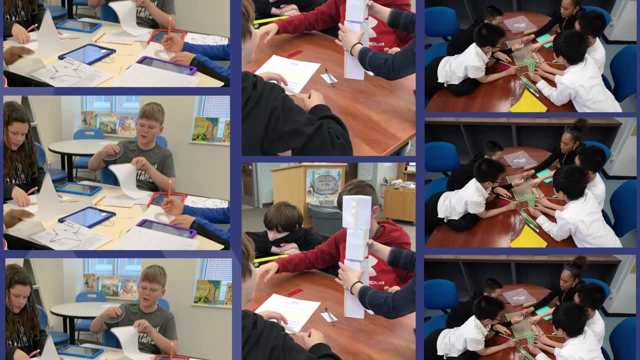 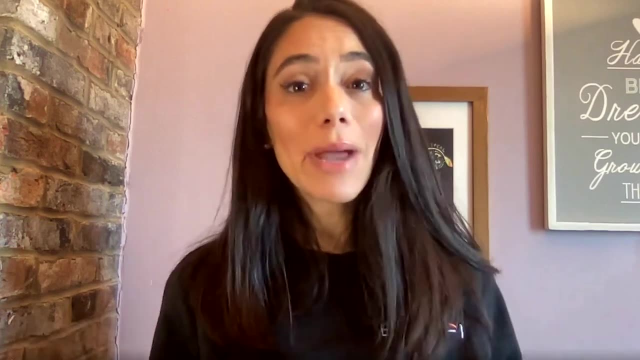 So have them actually go and see when they're ready, Make sure their muscles get tired, Work their endurance, See what that kinetic and potential energy looks like in real life. Go out and do a service project, Another one in the compassion project, where students actually go out and show compassion in their community. 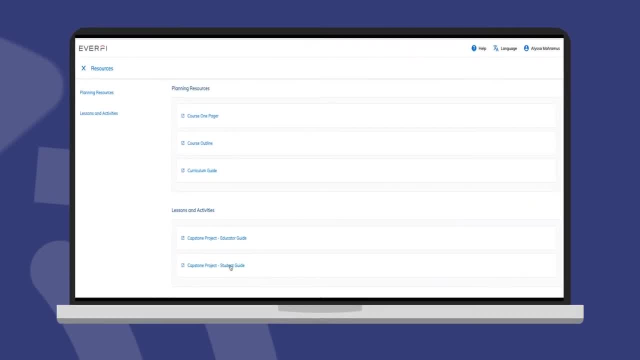 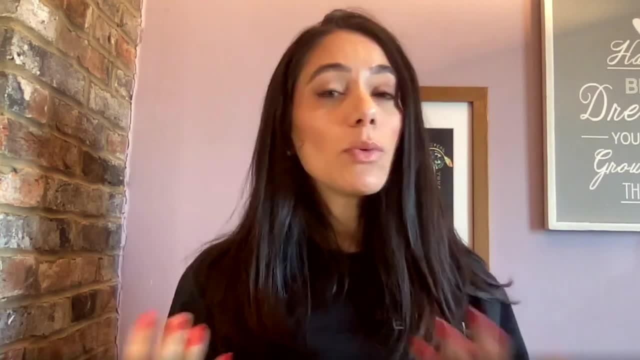 If you look at the Honor Code program, there's a whole capstone project where students are going out and being leaders in their community. It's a little bit more work on the teacher's end when you do a project, But with EverFi's resources.